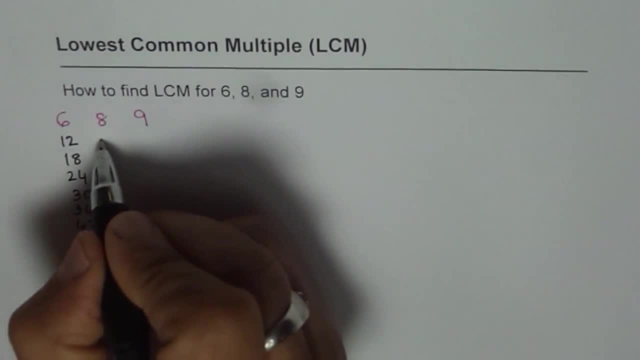 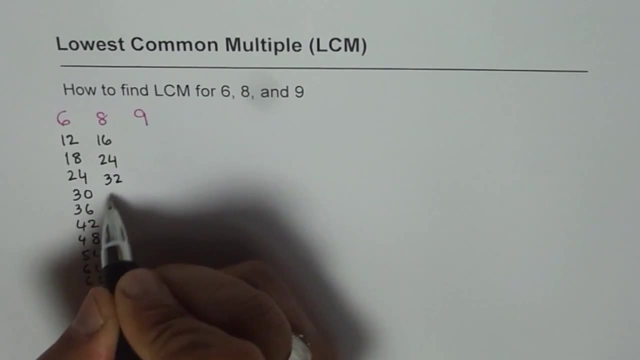 Let's start with 8.. For 8s we have: 8 times 2 is 16, then we have 24, and then we have 32,, 40,, 48.. 56,, 64,, 72,, 80.. 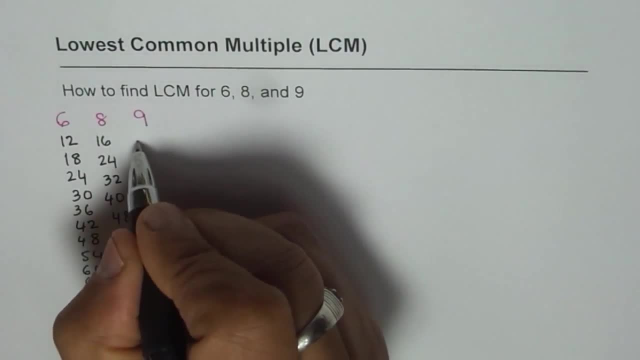 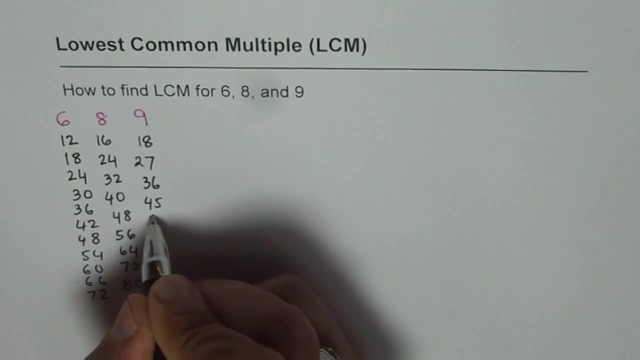 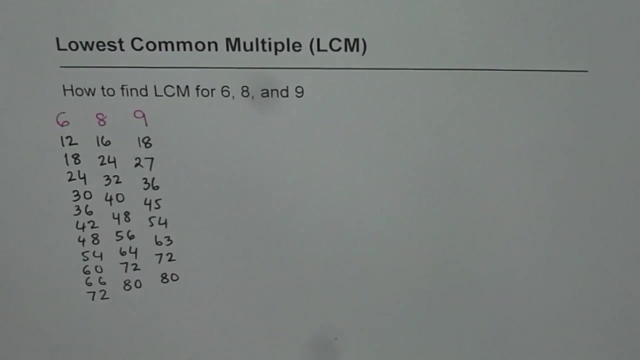 How about 9s? 9 times 1 is 9,, 9 times 2 is 18,, 27,, 36,, 45,, 54,, 63,, 72,, 80 and so on. Well, we already have a number. 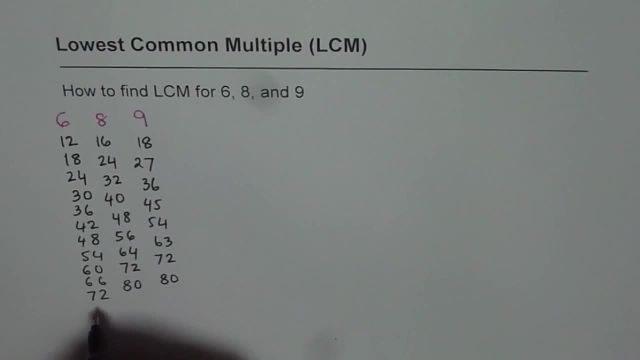 Well, we already have a number. We already have a number. We already have a number which is common to all right, which is 72.. So finding all the multiples can help you to find least common multiple right, but that may take a long time. 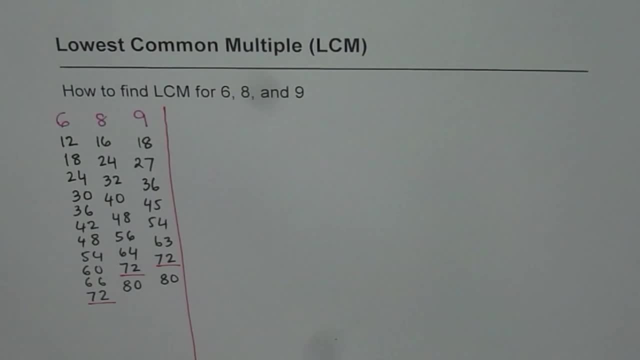 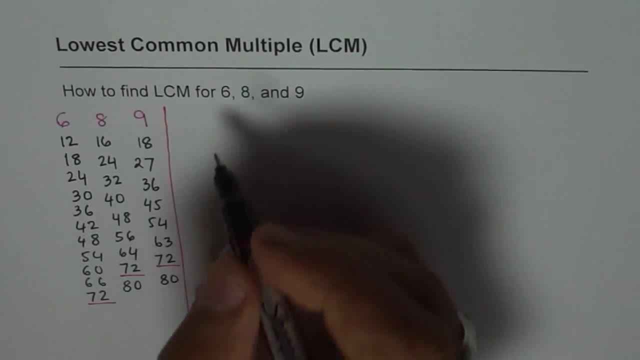 Okay, so that is one method. Well, we did get the answer, That's good. The other method is prime factorization. Let me show you that method now, which is 6, 8 and 9.. We are considering three numbers. 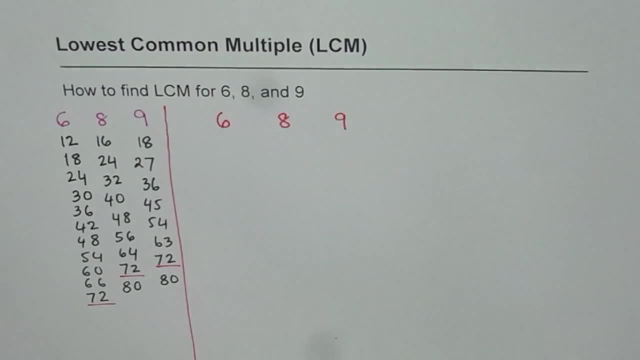 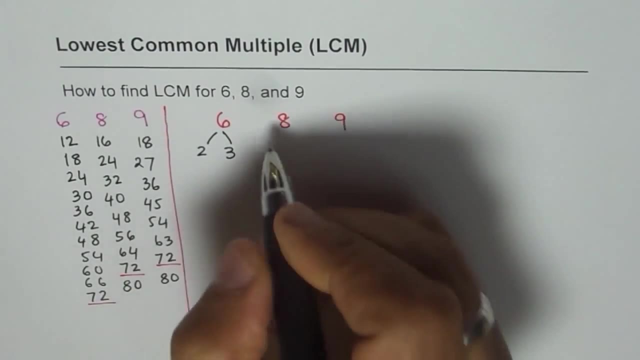 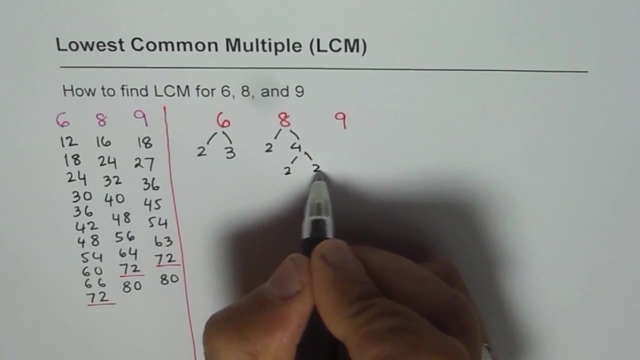 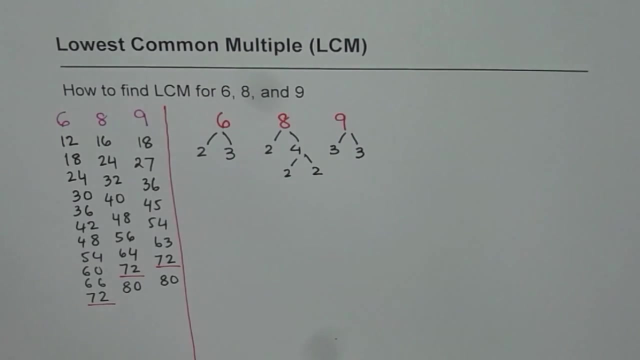 6., 8., 9., 8 and 9.. Let us find their prime factors. For 6, the factors are 2 times 3.. For 8, it is 2 times 4, and I can write 4 as also 2 times 2.. For 9, it is 3 times 3, correct? So we get factors of 6 as 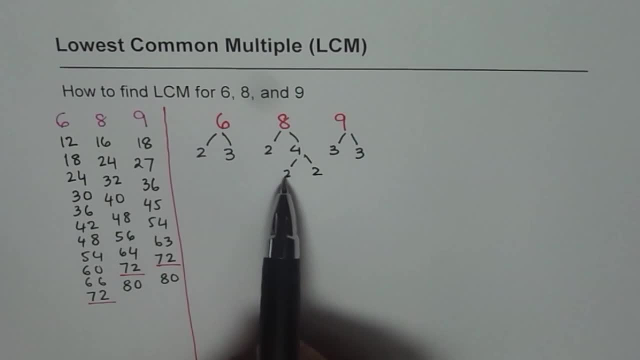 2 times 3, factors of 8 as 2, 2 and 2 and factors of 9 as 3 times 3.. Now to find least common multiple. what do we do? We see that there are two type of prime factors. One is 2s and the other. 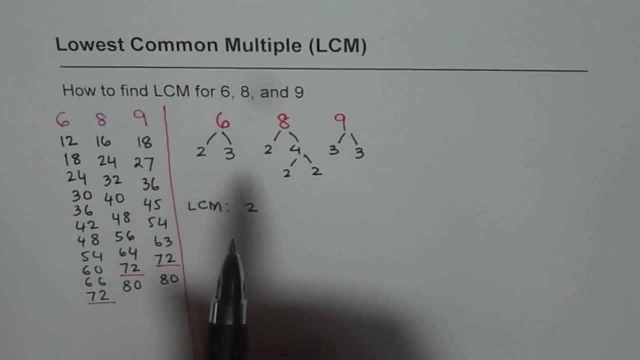 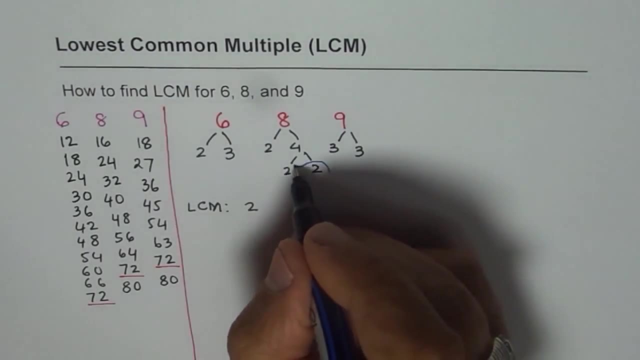 one is 3s. So what we do here is we check where are maximum number of 2s. So we find in 8, we have maximum number of 2s, There are 3 of them. So we will write down 3, 2s Multiply. 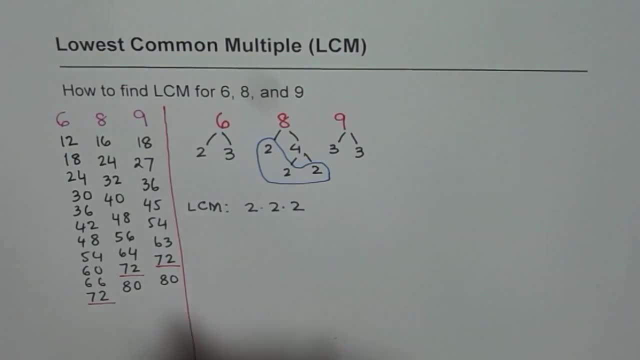 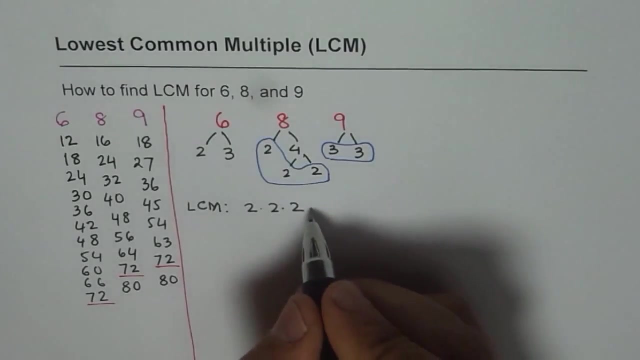 them together. Now. the second factor is 3s. We again see where are maximum number of 3s. We see, well, the maximum number of 3s are in 9, 2 3s. So we will write these 2 times 3.. So that gives you. 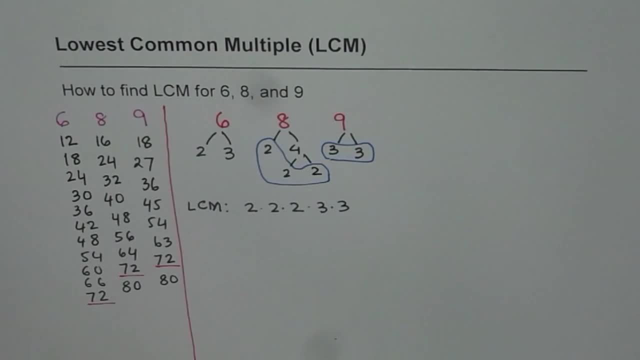 set of factors for our least common multiple right. Let's multiply them and get the answer. So the answer in this case is: 2 times 2 is 4, 4 times 2 is 8,, 3 times 3 is 9,, 8 times 9 is 72. 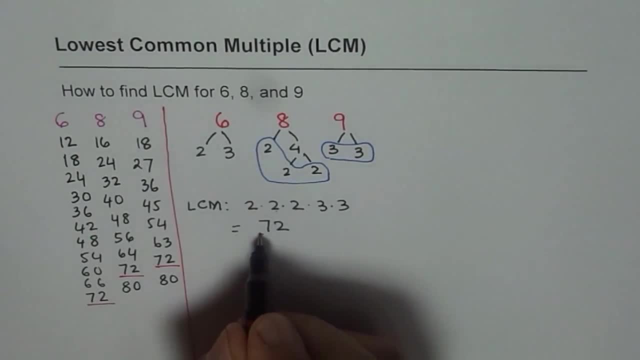 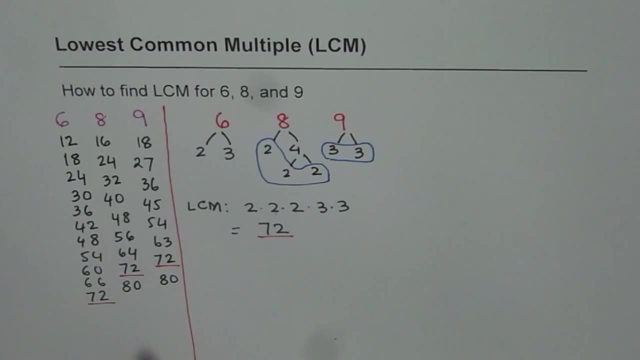 So you get the same answer. Do you see that? So you get the same answer: by prime factorization. Do you see that? So first, first step was: first method was using multiples. The second one we used is factorization prime. 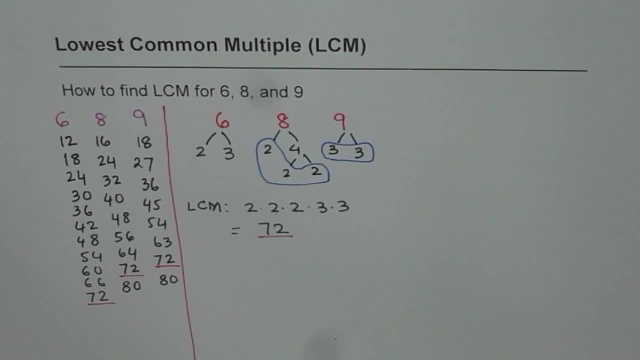 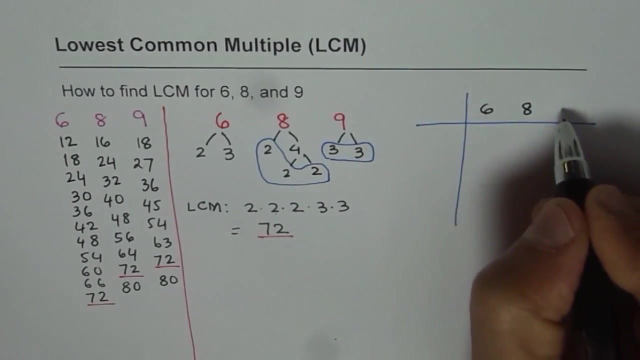 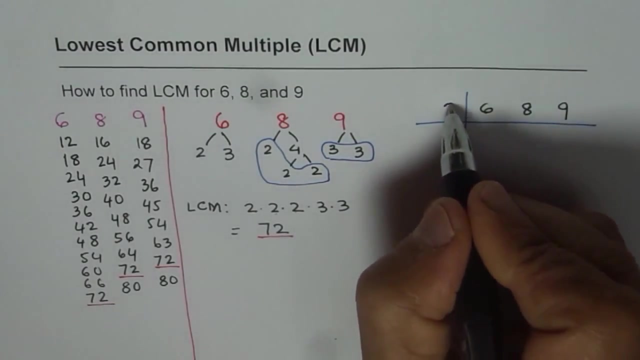 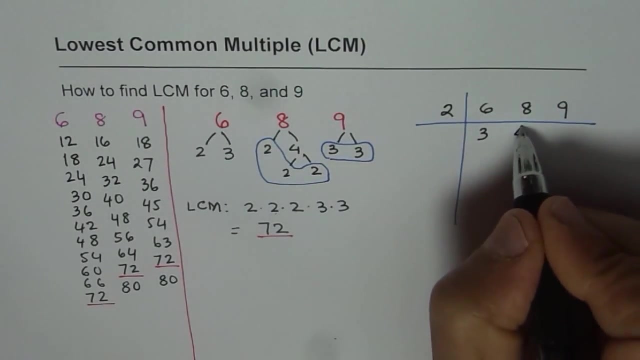 factorization. Now I will teach you another method of doing it, and that is by division. So what we do is we will repeatedly divide the numbers. We have three numbers: 6,, 8 and 9.. Now we can divide at least two of them by 2.. So if I divide 6 by 2, I get 3.. If I divide 8 by 2, I get 4.. But if I divide 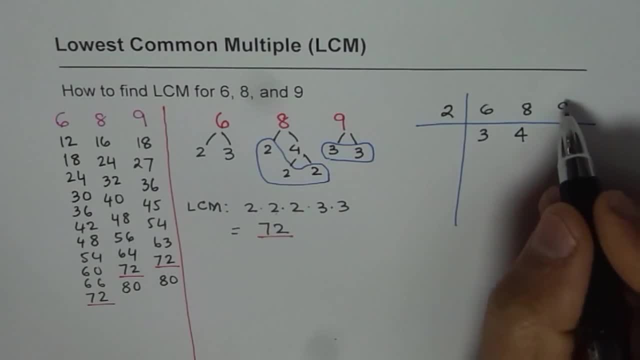 9 by 2, I do not get a whole number. So 2 is not a factor of 9.. So in that case I will just write 9 as such. Now we can divide at least two of these numbers by 3.. So 3 is a common factor. 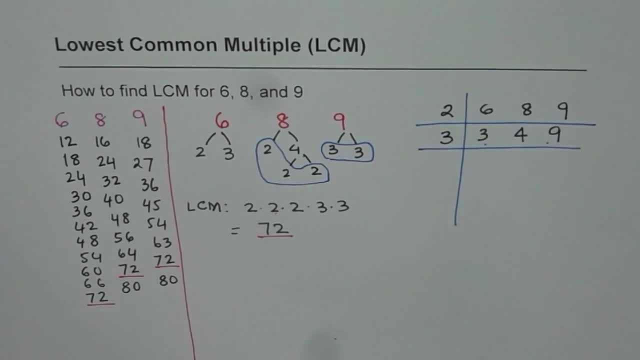 Therefore 2 of these numbers, and that is why we are dividing. Let's divide by 3.. 3, divide into 3 one time. 4, no 3 is not a factor, So we will write 4 as such And 3 goes in. 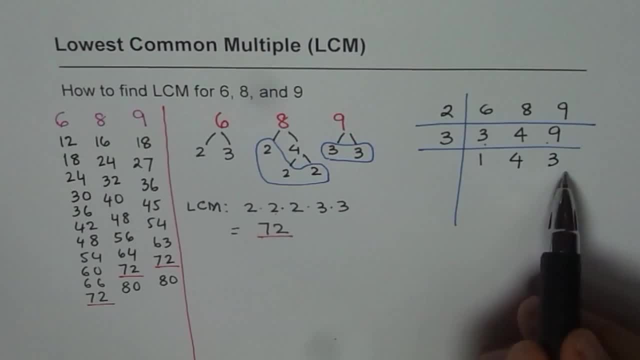 9, three times, So now 4 and 3, they cannot be divided by any common number And therefore that brings us to LCM, the least common multiple. So the least common multiple for us will be equal to product of these numbers, which is 2 times 3 times 4 times. 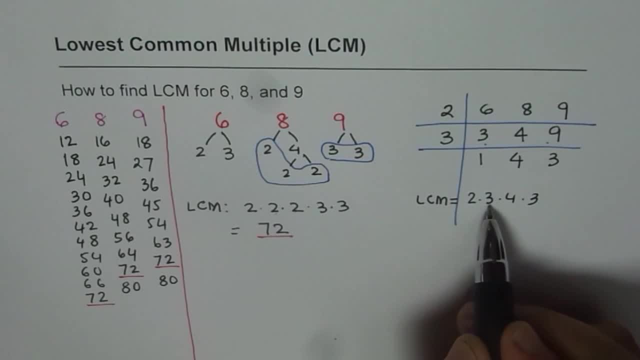 3.. 2 times 3 is 6.. 6 times 4 is 24.. And 24 times 3 is 72. So you again get the same answer, right? So that's the third method by which you get the same answer. Now let me show you. 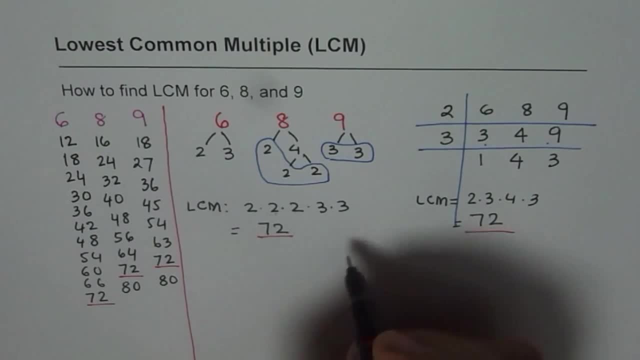 the fourth method also, And this time what I will do is I will make Venn diagram. So I am making for three numbers, three different circles. These are my three different circles. This is a very interesting method. Now, in these circles, I will write down all the factors of our numbers. So let 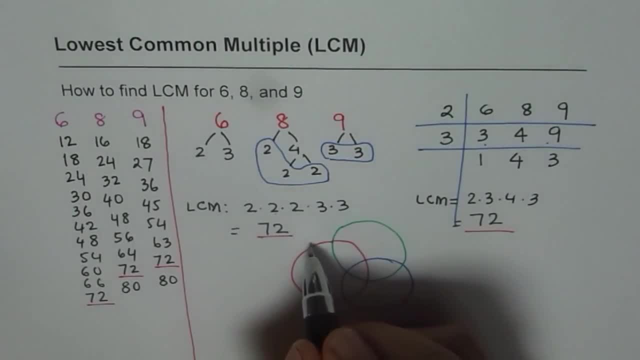 us say the first circle is for number 6.. Ok, So this one is for number 6.. Now for six, we have 2 and 3 as the common factor. And let us say this circle is for number 8.. And the last circle, the blue one, is for: 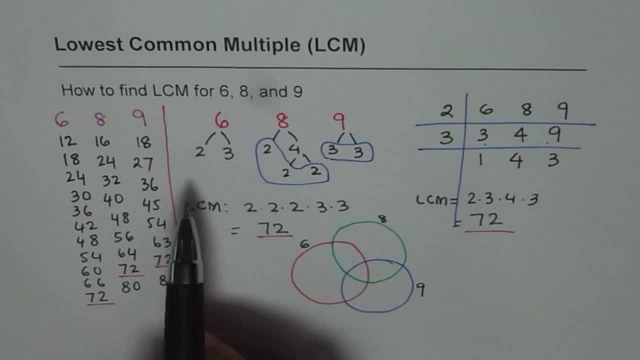 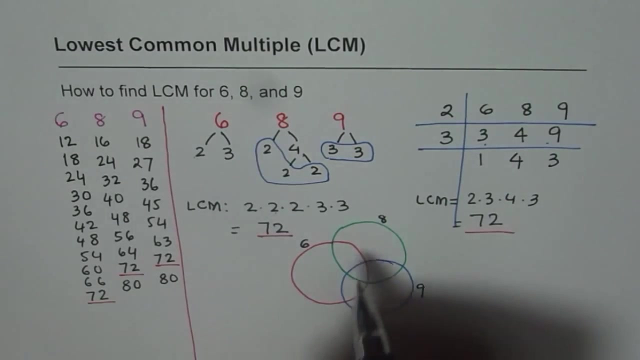 number 9.. Now, there are two factors of 6 – 2 and 3,. but 2 is also a factor of 8,, right? So what I can do is I can write this: 2,, which is common to both 6 and 8, right? so 6 and 8 common to, will write here. as far as 3 is concerned, 3 is: 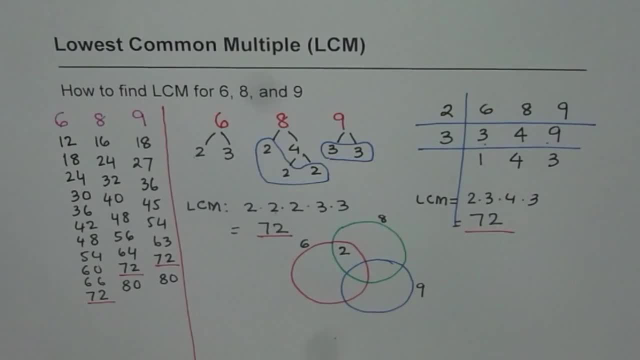 common with 9, right? so what I will do is I took this 2 as common with 8 and I wrote it here. now the other 2, other 3, I should say 3- is common with 9, so where should I write it? it is common. 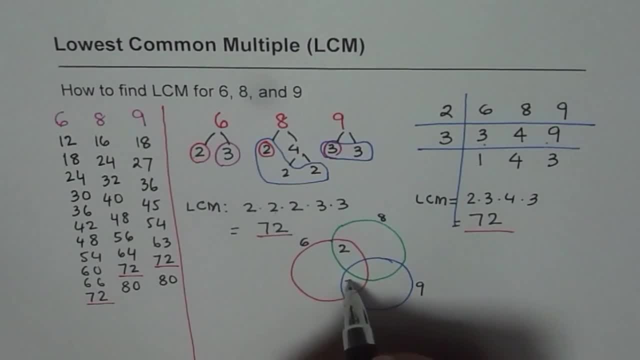 to 6 and 9. between 6 and 9, I will write 3 here, so I've taken care of 2 and 3. as far as 8 is concerned, we have already taken care of 1- 2, but there are 2, 2s which are left, so I'll write these 2s here. 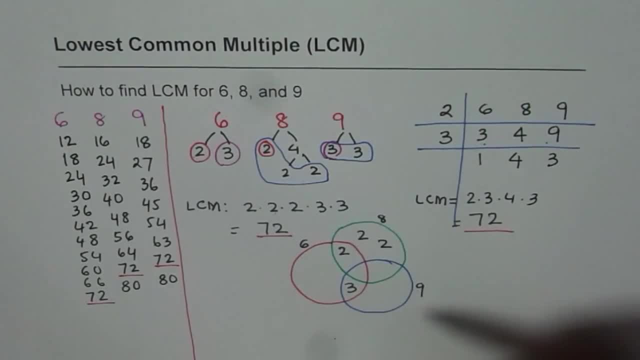 in 8. now, as far as 9 is concerned, we have already taken 1, 3. 1, 3 is left. I will write it here now you can check. as far as 6 is concerned, the red circle we have 2 times 3 as 6- 8. the green circle we have 2 times. 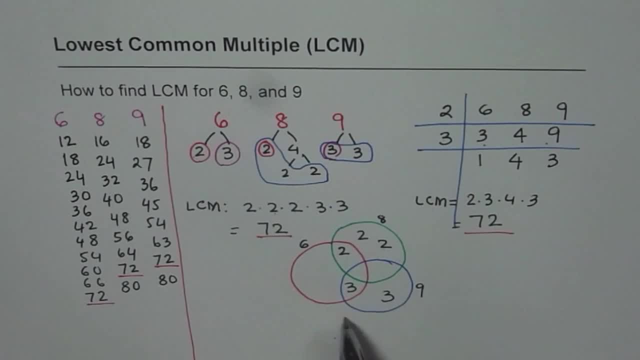 2 times 2 as 8 blue circle is for 9. 3 times 3 is 9, right? so we got all the factors in the Venn diagram. do you see that? so that is my Venn diagram. okay, so this is using Venn diagram. 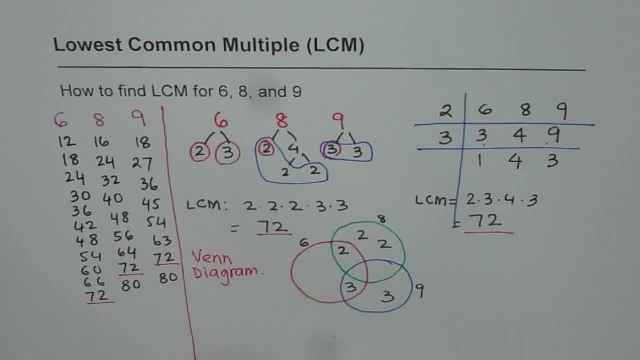 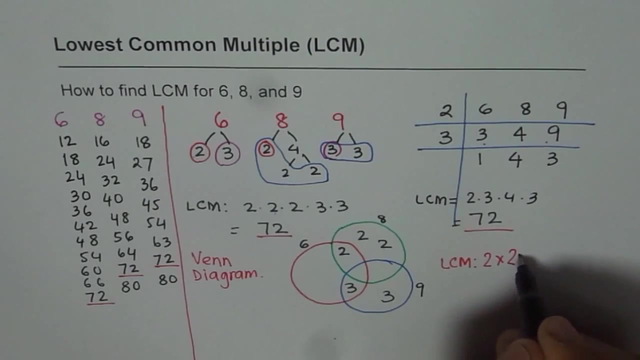 now, can you tell me what is the LCM using this Venn diagram? LCM is product of all these numbers, so let's multiply them. what do we get? 2 times 2 times 2? these are 3, 2s. and then we have to do these two 3s right. what do we get 2 times 2, 4. four times 2, 8. 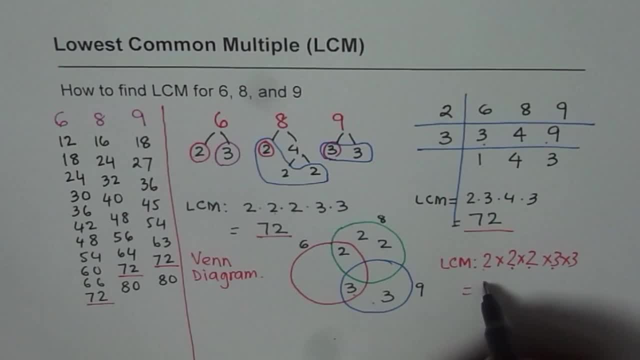 8 times 3, 24, 24, 3, 7, 7, 52. So we get the same answer. Do you see that? So in this video you have learned four techniques to find lowest common multiple. The first one is just list all the multiples. 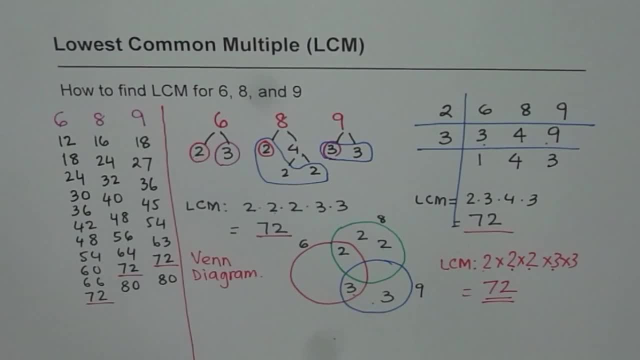 find the lowest common. Second one is prime factorization. right In prime factorization, find the prime factors and pick up the ones which has maximum of that type. Then we had repeated division. In repeated division, keep on dividing by common factors for at least.